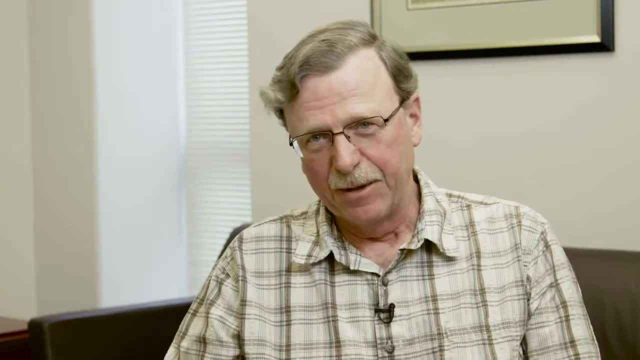 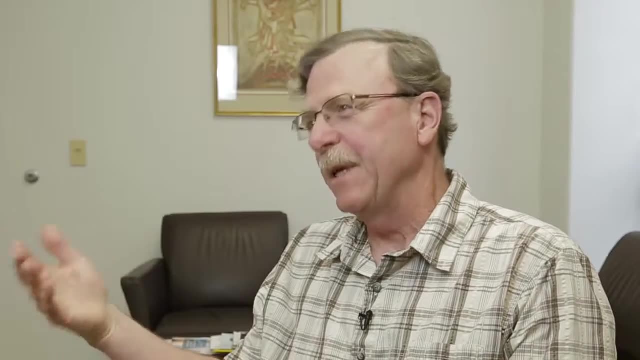 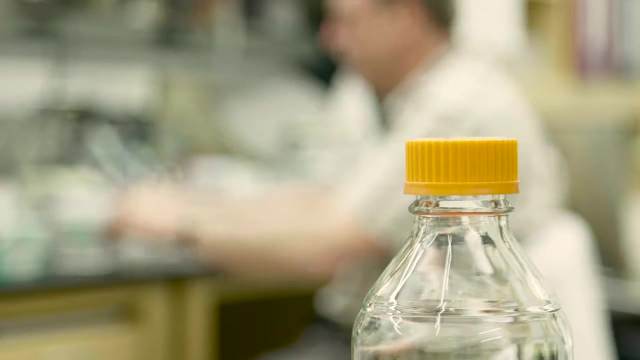 And so over the years we've been involved in multiple studies and other labs have as well, trying to understand exactly how that protein DNA complex really messes cells up and how they try to respond to it, And that's work that's still ongoing in a number of labs. 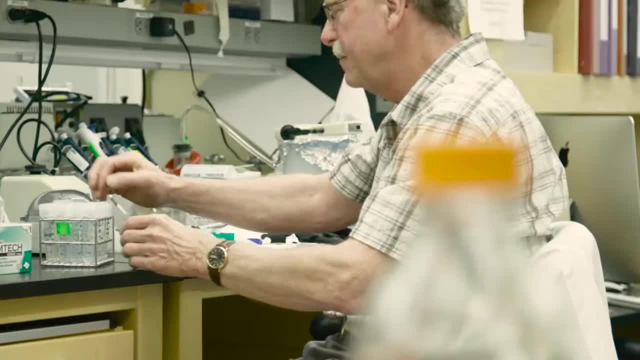 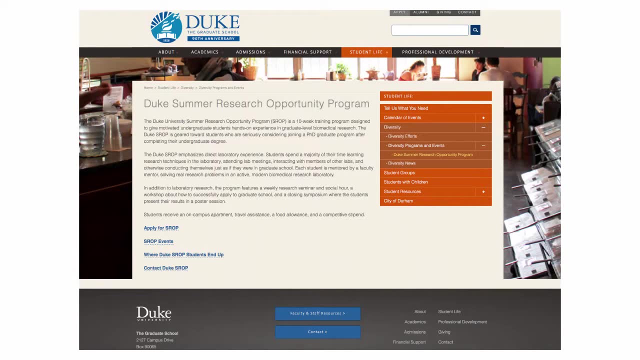 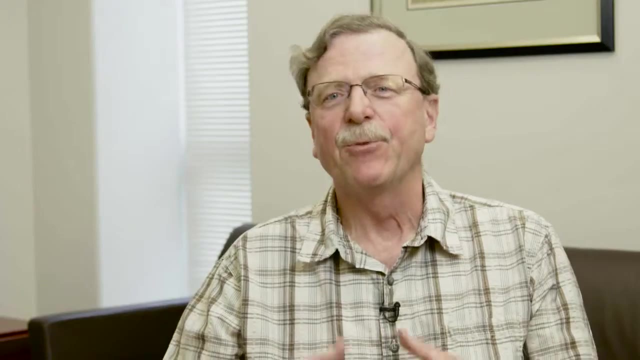 Away from the bench. Kruiser has been a passionate advocate to attract more underrepresented minorities to the medical sciences. He pioneered Duke's Summer Research Opportunity Program, which is now more than 20 years old, And we've trained well over 200 students in the program. We give them research opportunities. 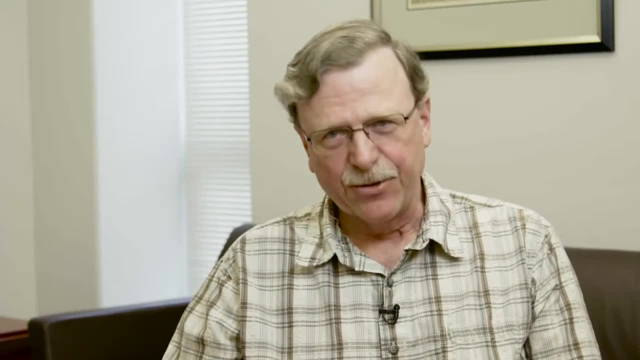 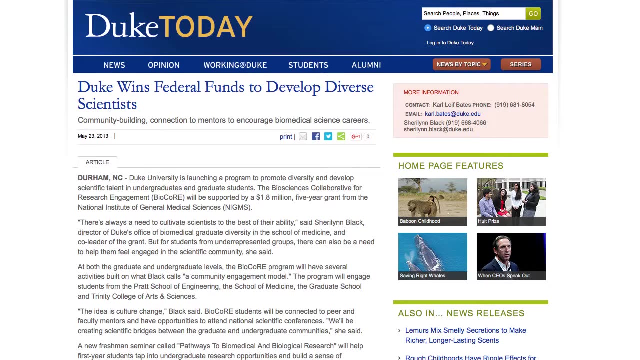 for 10 weeks in the summer and also a lot of seminars about career development and things like that. Along with Sherrilyn Black and Julie Reynolds Kruiser, co-created a program called BioCore, which is partially funded by the NIH to support undergraduate and graduate research for underrepresented 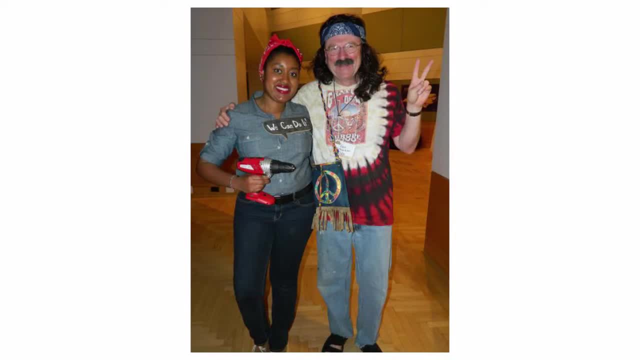 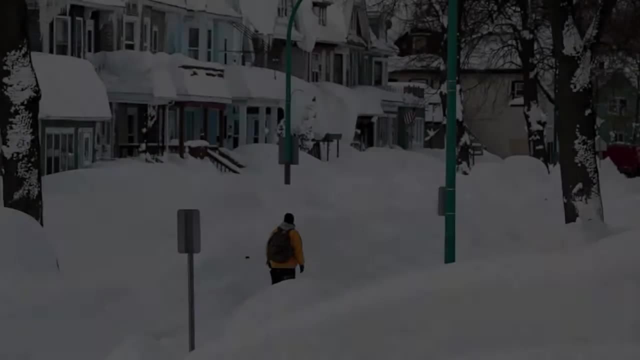 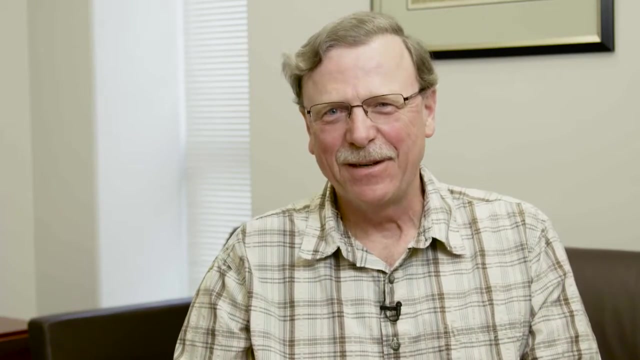 minorities And it's just been incredibly rewarding to see, you know, hundreds of kids, really, you know, getting to experience science. Kruiser was raised in Buffalo, New York. before heading off to college It was pretty miserable up there, after about five months of snow and cold. 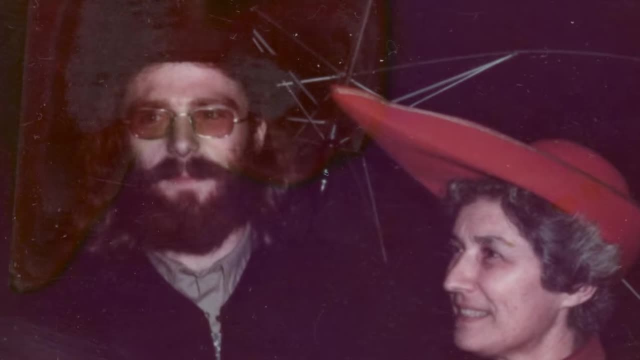 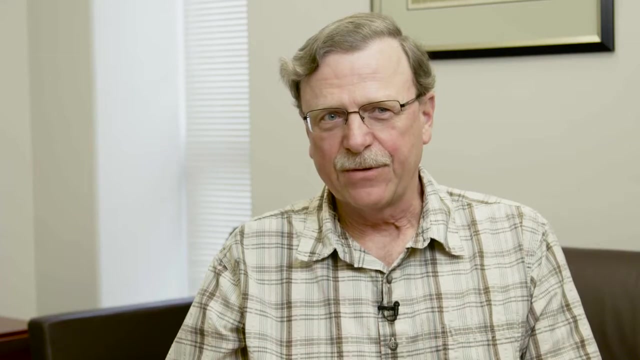 He has always been interested in science and it was as an undergrad at MIT where he was bitten by the research bug. And what was then? the research bug? The new field of molecular biology. I took a course from a guy named Salvador Luria who got the Nobel Prize, actually. 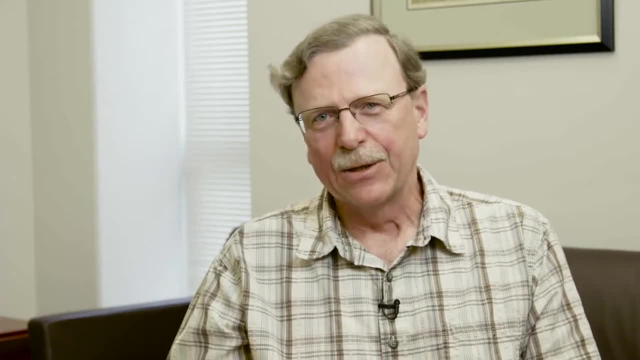 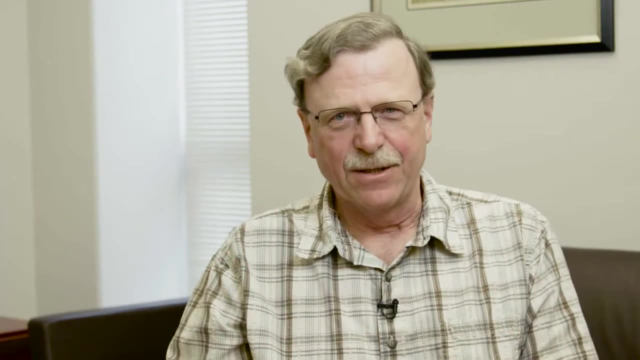 And he was just absolutely inspirational, showing how you could learn about what's going on with the DNA molecule by looking at the color of colonies on petri plates, And so in that course I kind of learned that it was actually possible to figure out things. 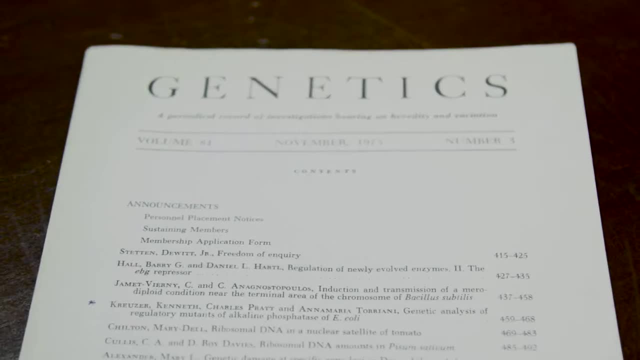 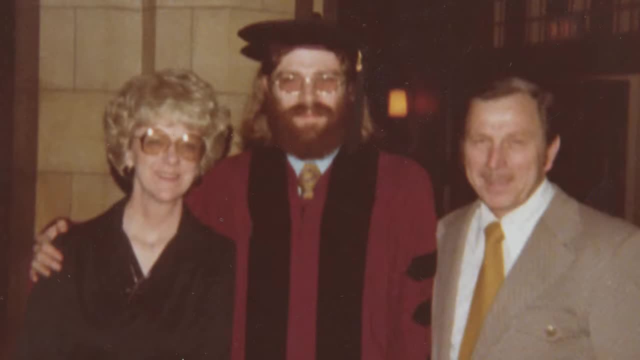 about how life works at the molecular level. It was also at MIT where he had his first paper published on the topic of gene regulation in Syria. He earned a PhD in genetics at the University of Chicago and came to Duke in 1984 after. 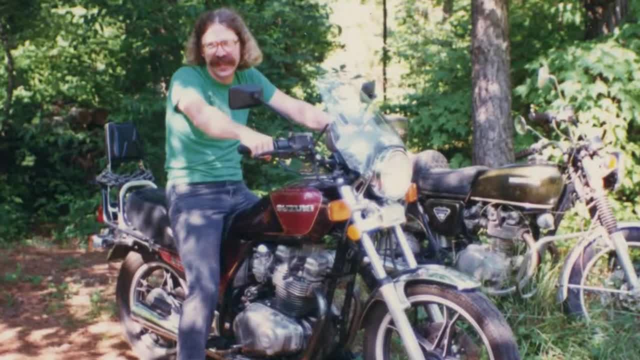 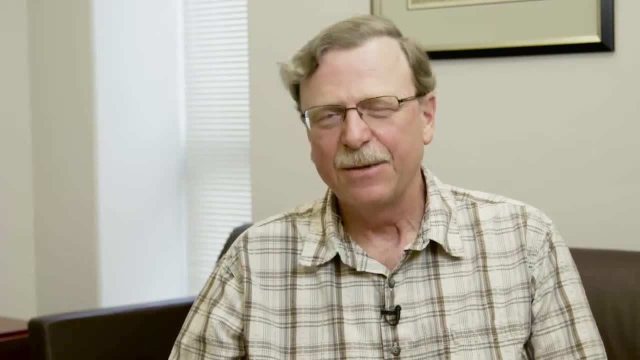 fellowships in Chicago and the University of California, San Francisco, And what I found at Duke was, you know, I could sense there was the opportunity to do good science And it seemed to be on the upward trajectory, which certainly turned out to be true over.